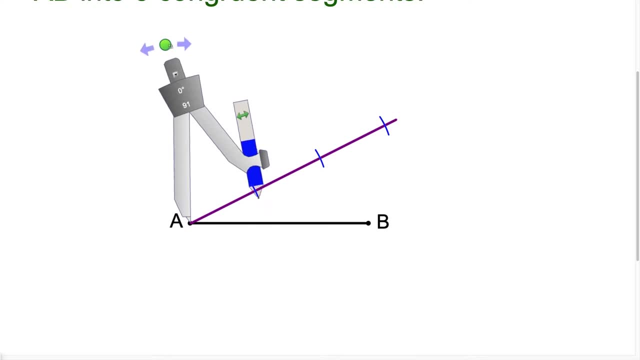 from here is: I'm going to set the compass on point A and I'm going to measure the length of this entire segment, So all three of them together like this, And now, just to make sure that I set it to a good amount, you see that drawing goes right. 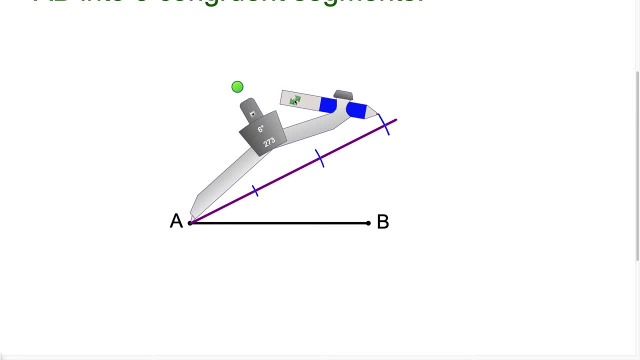 over itself. So I know that's a good distance to set it to. So now I'm going to move the compass over from A to right in the middle of point B and I'm going to swing an arc, And what I'm essentially doing is I'm going to be building a line segment equal in length. 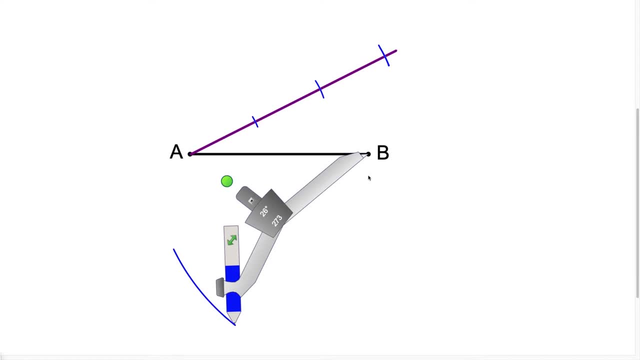 to this purple one and I need it to go from B and it's going to go through this arc that I just made, But just to make sure that I'm drawing it in the accurate spot. the next thing I need to measure here is I need to measure the distance from B to this last point over here on the. 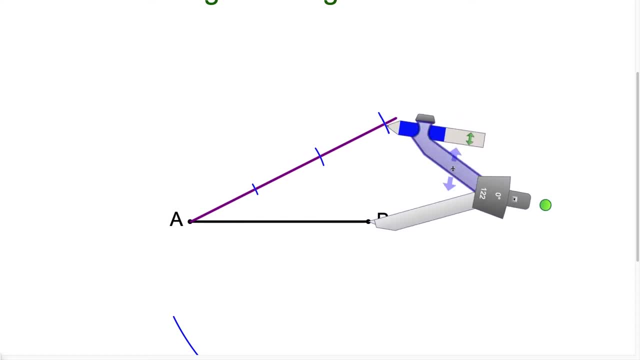 purple line segment. So extend it over here like this, maybe go out a little bit further and we'll see this one here lines up pretty well with the purple line. So now that distance I'm going to keep and I'm going to move it over to point A. 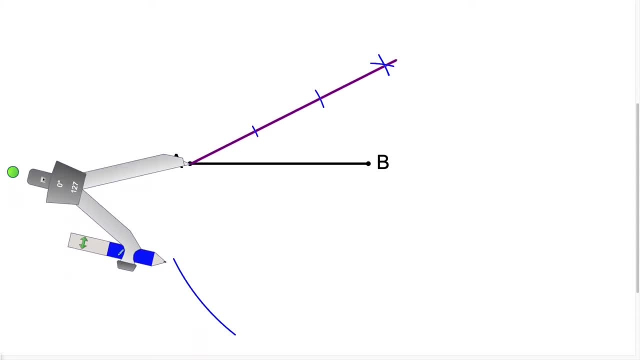 And from here, what we want to do is we want to place the compass on A and we're going to swing an arc like this and notice that this arc intersects the one we just made before. So now I'm I'm going to draw in my line and I'm coming in from point B and I'm going to draw it. so 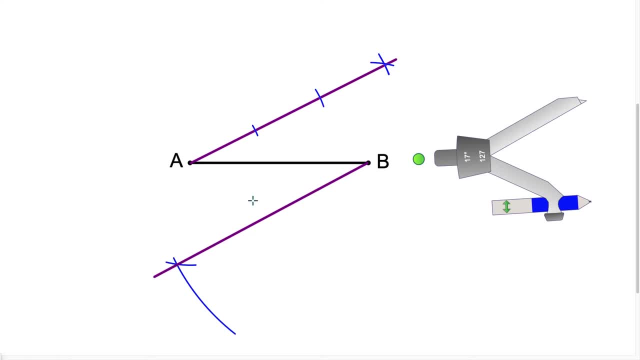 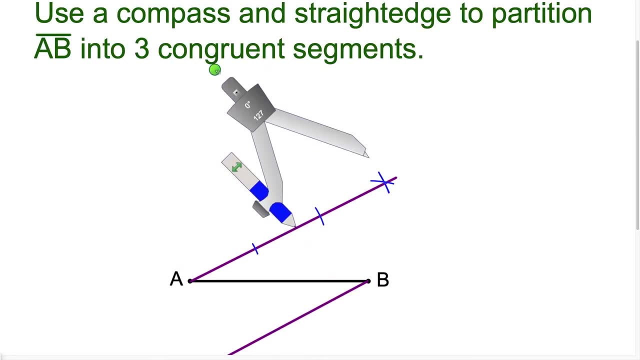 that it intersects the intersection of those two arcs. Now one of the last steps I need with the compass here is I have to go back to the original purple line segment here and I need to measure that initial amount. So notice the segment here. all three of them were equal in length. 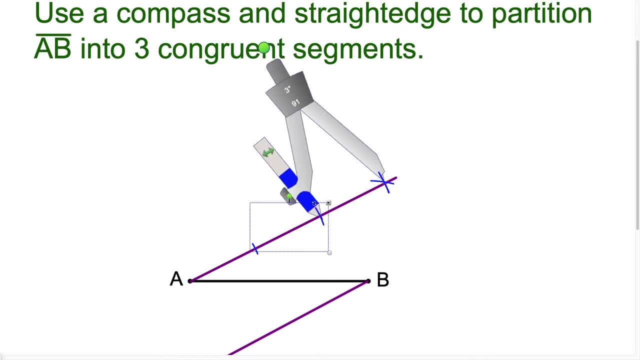 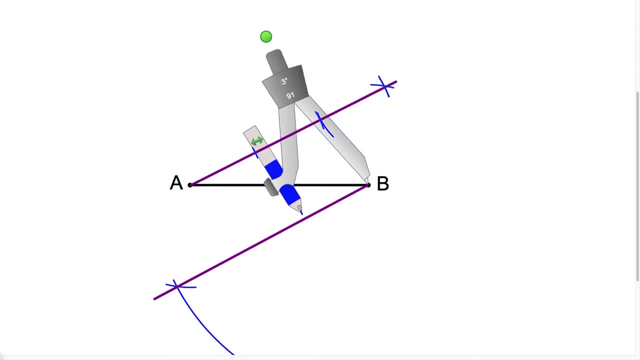 So I could just measure it to be set to one of them, And what I'm going to do here is I'm just going to draw this in to show that I'm measuring it and I'm setting the compass on point B, And now I'm going to make the same three marks like this: 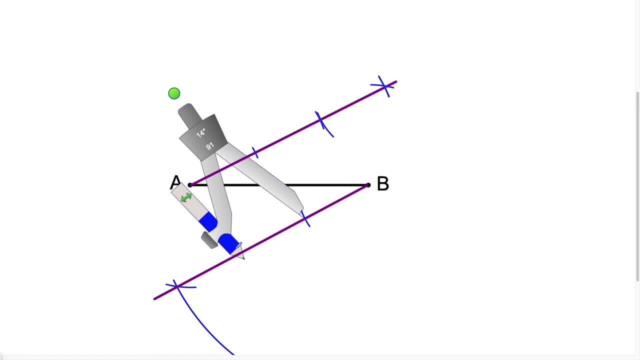 So I have one, the second one is over here and then, if we look here, the third one should line up nice with what we just drew, and you could see it lines up pretty well with the last one we just drew. So then the last step here to this construction is- I'm just going to connect this point to 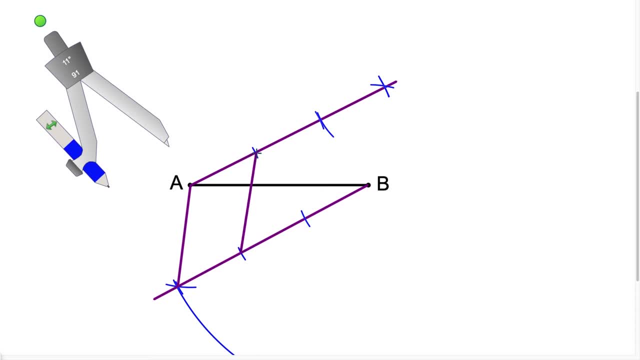 this point here and then I'm going to connect this point here with this one. So notice, I got one, two, three, four points to connect and essentially what we did was just construct a parallel, The parallelogram. the opposite sides were cut at specific locations, so these three segments-